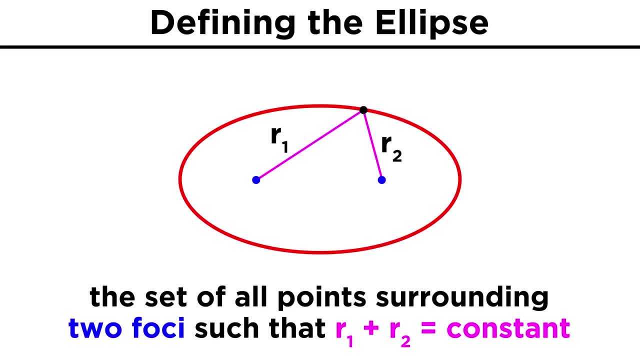 the distance from a point to one focus plus the distance from that point to the other focus is constant. No matter what point we are looking at on this ellipse, the sum of these two distances will be the same: As it gets closer to one, it's farther away from the other, and vice versa. 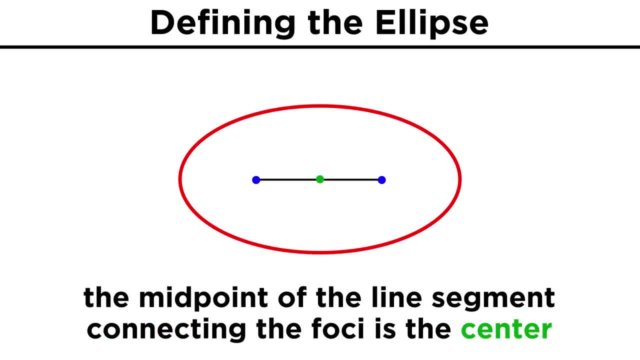 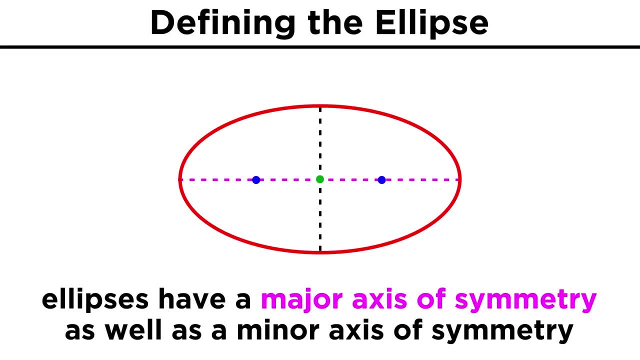 The midpoint of the line segment that connects the foci is the center of the ellipse. Ellipses also have two axes of symmetry: a major axis, which will be the longer one, and a minor axis, which is the shorter one. At each end of the major axis we can find a vertex, and that's all the terminology. 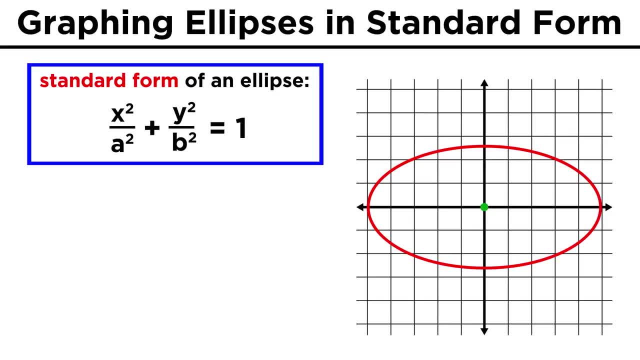 we need to know. The standard form of the equation of an ellipse that has its center at the origin looks like this: It's similar to the equation for a circle, but we have these terms A and B, which give us information about the major and minor axes. 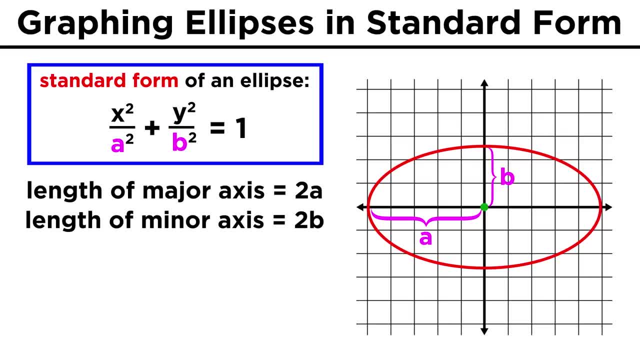 Specifically, the major axis has a length of two A and the minor axis has a length of two B, or we could think of A as the distance from the center to a vertex. If we solve for C, that is the distance from the center to either of the foci. 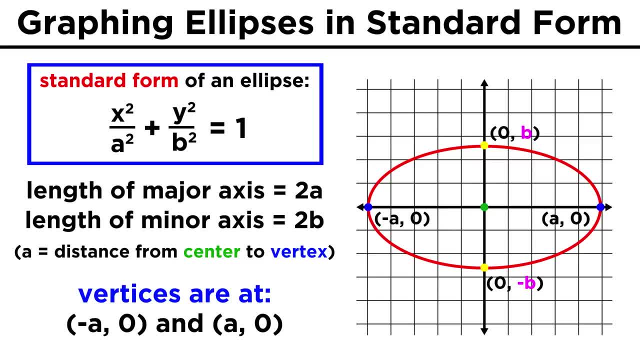 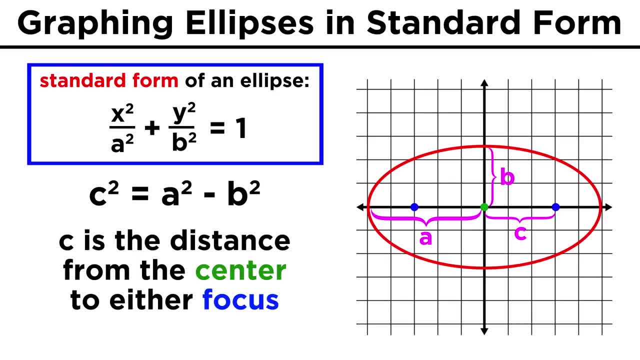 On the major axis, which means that positive and negative A are the X intercepts and positive and negative B are the Y intercepts. Beyond this, we can use this equation: C squared equals A squared minus B squared, and if we solve for C, that is the distance from the center to either of the foci. 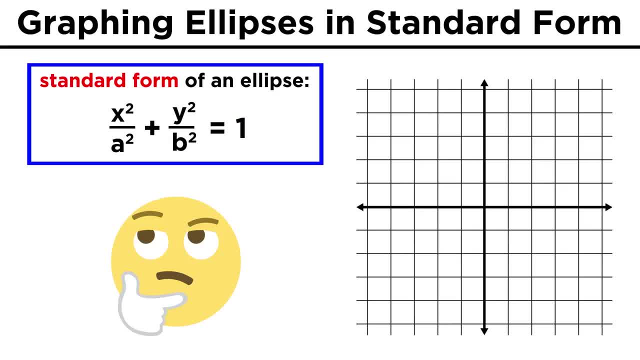 It's one over here. it's very easy to graph it. Say we have a nine for A squared and a four for B squared. That means A is three and B is two. so we would just draw the four intercepts connect. 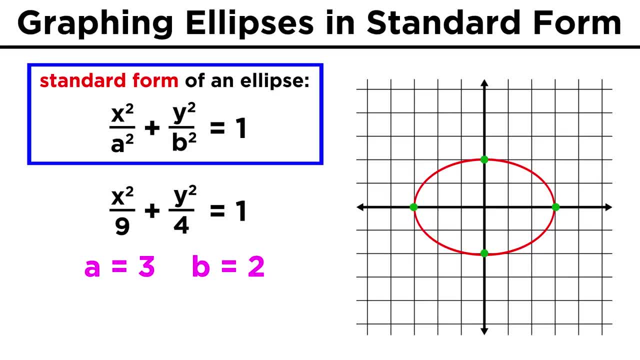 them, and there's the ellipse. The foci are not part of the ellipse, but if we need those as well, that will come from C squared equals nine minus four, Or C equals plus or minus four, And that's it. Minus root: five. 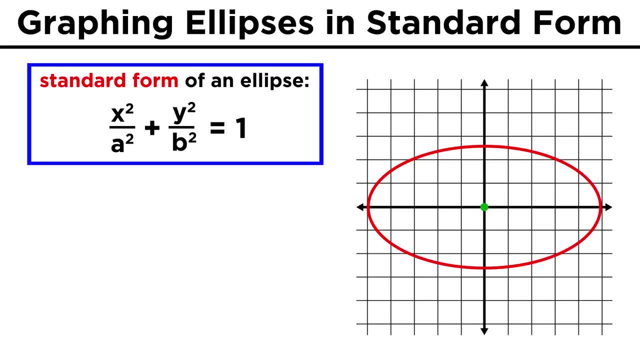 The standard form of the equation of an ellipse, that has its center at the origin, looks like this. 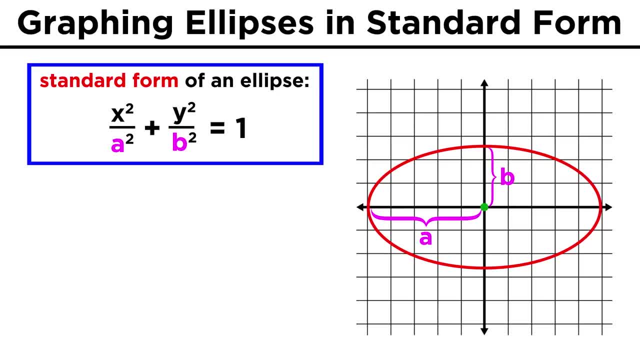 It's similar to the equation for a circle, but we have these terms, A and B, which give us information about the major and minor axes. Specifically, the major axis has a length of two A, and the minor axis has a length of two B, or we could think of A as the distance from the center to a vertex. 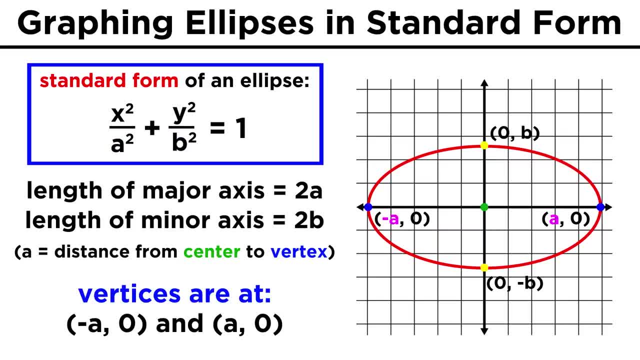 In today's case, we're only going to use the major and minor axes, but we're also going to say that the major and minor axes have a distance from each other. So we can say that they're both the same. In the standard form of the ellipse, the center is the 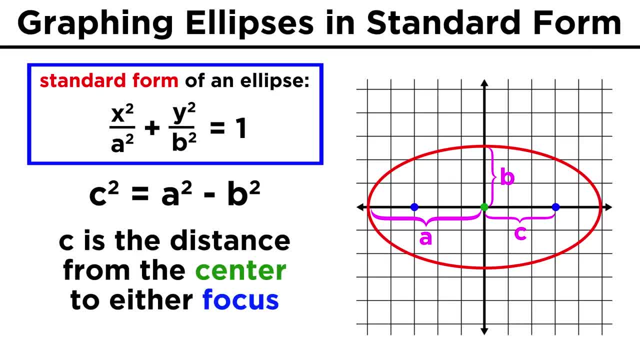 ivotal axis, so it's a position that looks like this. It's also the center of the force's strength. So if we add up all the two points, we're going to get the positive and negative A on the major axis, which means that positive and negative A are the X intercepts, and positive and negative B are the Y intercepts. Beyond this, we can use this equation, C squared equals A squared minus B squared, and if we solve for C, that is the distance from the center to either of the foci. 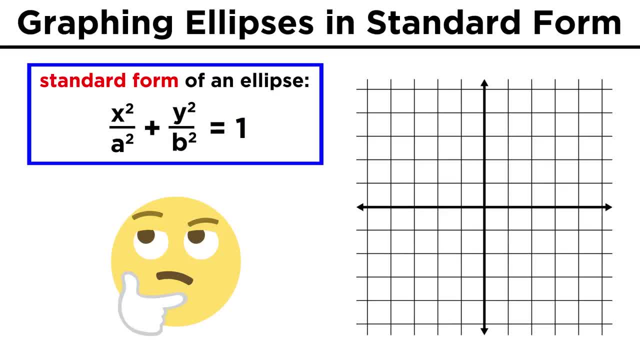 equation in standard form, with a one over here, it's very easy to graph it. Say we have a nine for A squared, and a four for B squared. That means A is three and B is two, so we would just draw the four intercepts, connect them, and there's the ellipse. 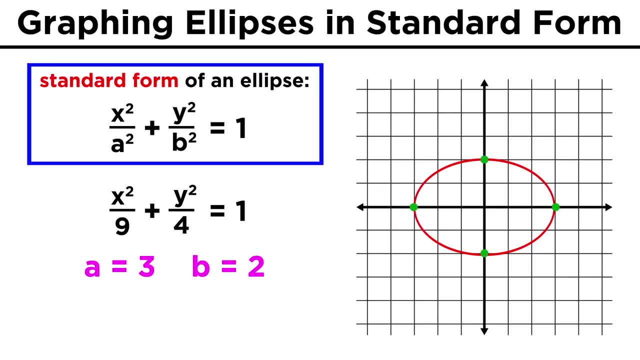 The foci are not part of the ellipse, but if we need those as well, that will come from C squared equals nine minus four, or C equals plus or minus root five. We should note that A is always greater than B, so if the term below X squared is greater than the term below Y squared, we have A here and B here, which produces an ellipse that is wider than it is tall. 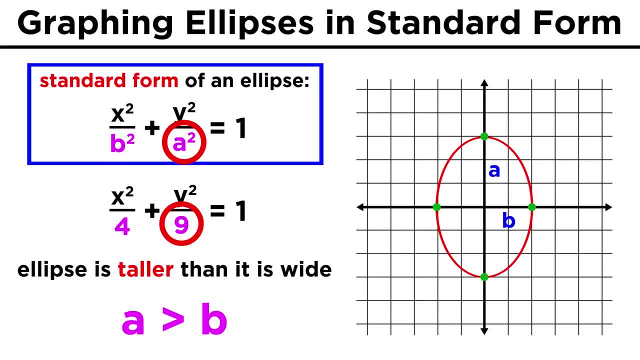 But if the other number is larger, then this term is A squared and this other term is B squared. 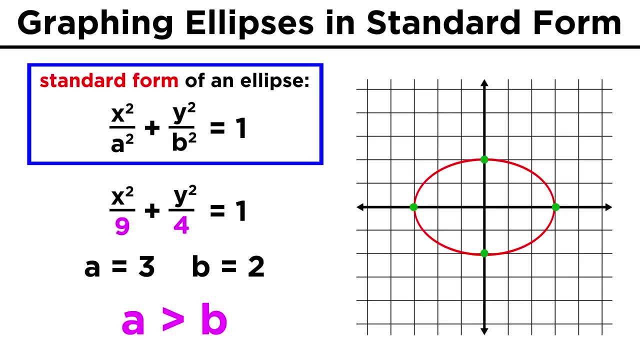 We should note that A is always greater than B. so if the term below X squared is greater than the term below Y squared, we have A here and B here, which produces an ellipse that is wider than it is tall. But if the other number is larger, then this term is A squared and this other term is 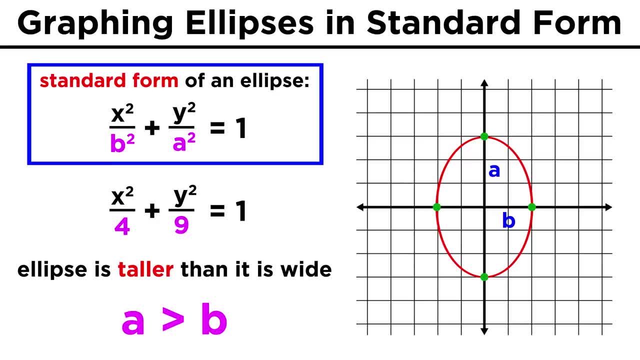 B squared. This is because the ellipse will now be taller than it is wide, But the A term must always correspond to the major axis, which is the longer axis, so that will now be the vertical axis given by Y. Let's say we have an equation for an ellipse where this number doesn't equal one. 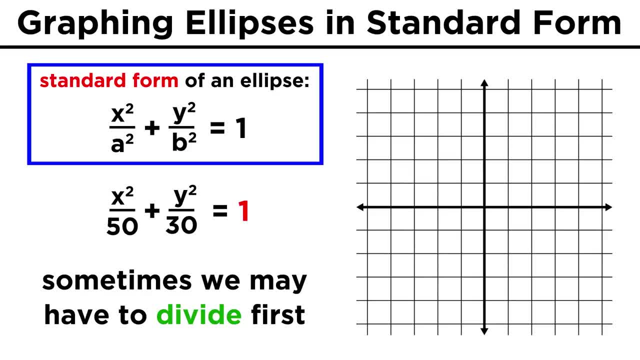 We will have to divide the entire equation by this term so that we get a one on this side, as it will be easier to graph in standard form, even if we end up with weird numbers for A and B. We could also graph an ellipse, with an ellipse in the center of the box. 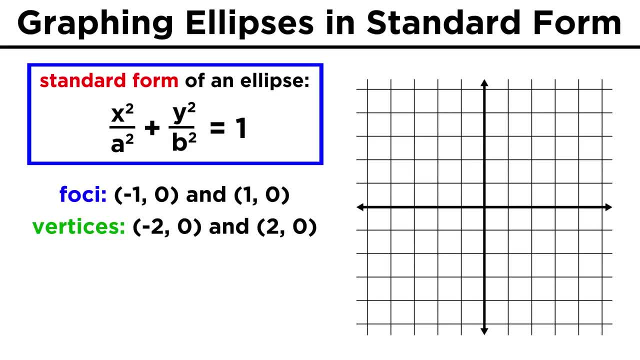 if we were to do an ellipse with a square under it, then we'd have to divide the whole number by that number so that we get a one on this side, as it will be easier to graph in an ellipse if given information about its foci and vertices. 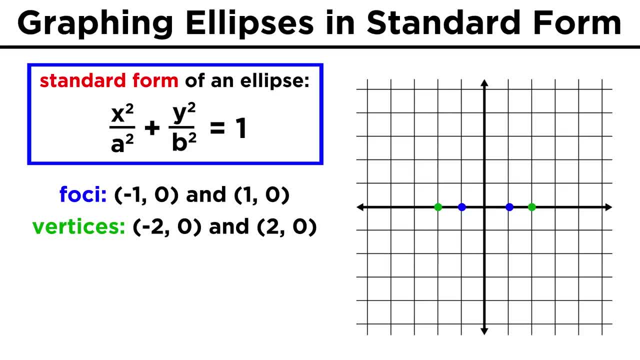 Say, the foci are at plus and minus one, while the vertices are at plus and minus two. That means that C is one and A is two. It will then be true that one equals four minus B squared, or B squared equals three. 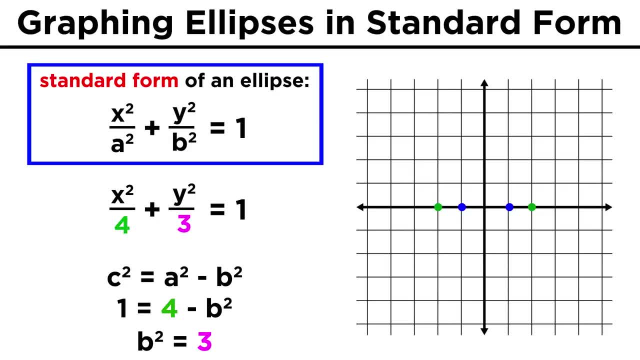 Then we just put A squared and B squared into the standard form, and there's our equation. Ellipses can be transformed by some of the ways we already know, except in this case. We can write X minus H, quantity squared, and Y minus K, quantity squared, rather than X squared. 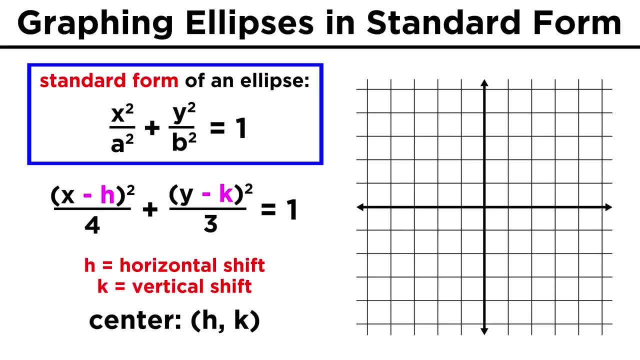 and Y squared and these H and K values will be the horizontal and vertical shifts respectively. Notice the minus signs. So X minus two will mean a shift of two to the right, not left. When we have H and K terms, the ellipse has a center at the point HK and everything else. 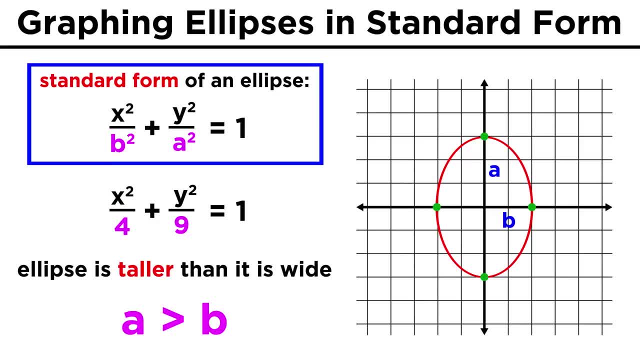 This is because the ellipse will now be taller than it is wide, but the A term must always correspond to the major axis, which is the longer axis, so that will now be the vertical axis given by Y. 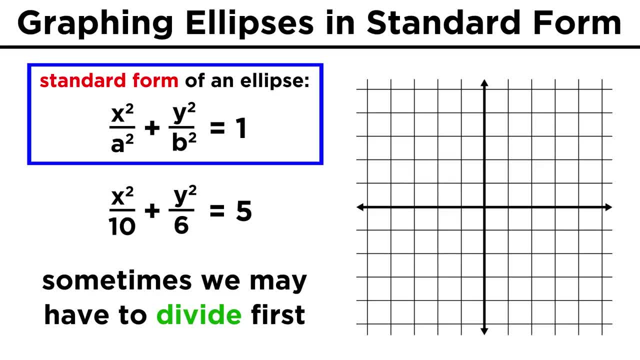 Let's say we have an equation for an ellipse, where this number doesn't equal one. We will have to divide the entire equation by this term so that we get a one on this side, as it will be easier to graph in standard form. 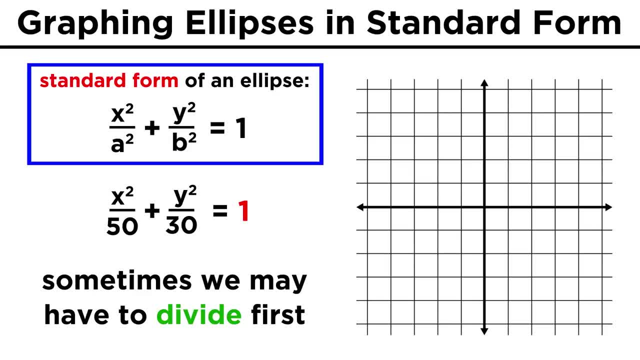 Even if we end up with weird numbers for A and B. 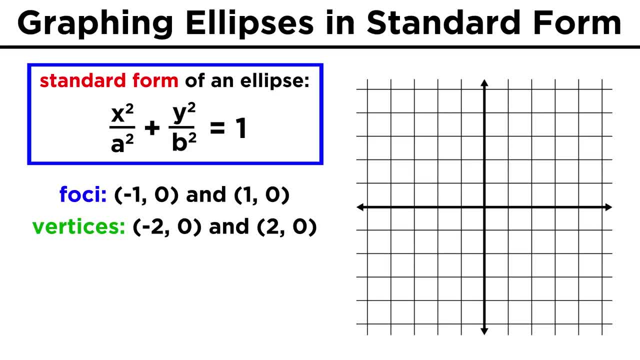 We could also graph an ellipse if given information about its foci and vertices. Say the foci are at plus and minus one, while the vertices are at plus and minus two. That means that C is one and A is two. It will then be true that one equals four minus B squared, or B squared equals three. Then we just put A squared equals B squared. That's the only way to do it. So let's put A squared and B squared into the standard form, and there's our equation. Ellipses can be transformed by some of the ways we already know, except in this case. We can write X minus H quantity squared and Y minus K quantity squared rather than X squared and Y squared, and these H and K values will be the horizontal and vertical shifts, respectively. 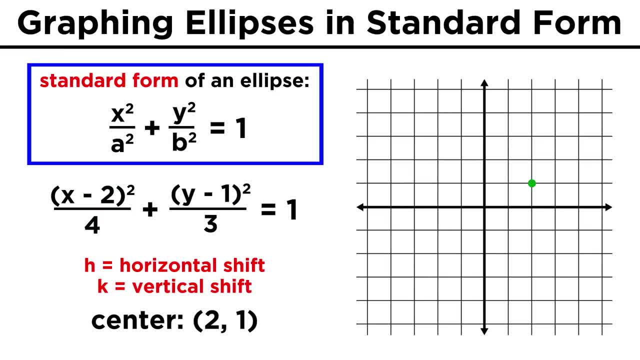 Notice the minus signs. So X minus two. X minus two will mean a shift of two to the right, not left. 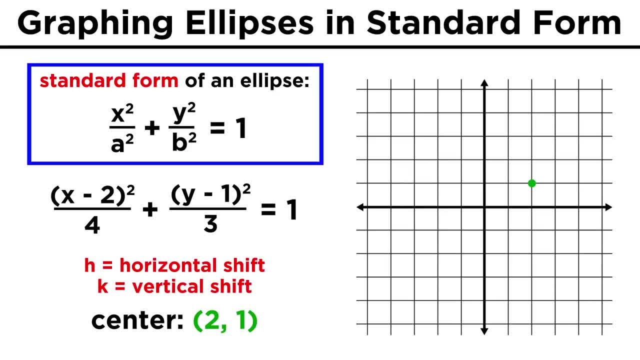 When we have H and K terms, the ellipse has a center at the point HK, and everything else we learned about the axes and foci will stay the same. 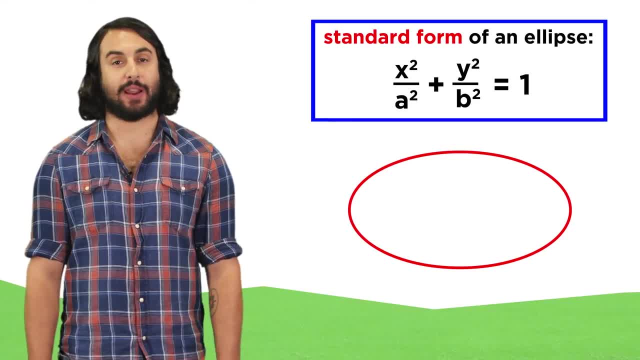 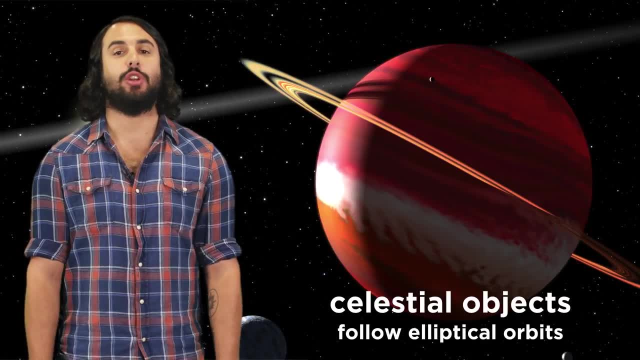 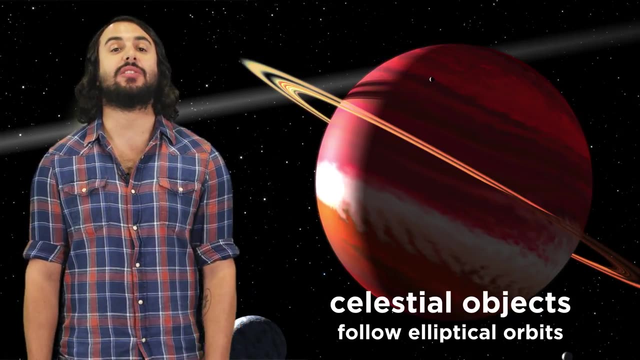 That's really all we need to know about ellipses right now. These are extremely important shapes for astronomy and astrophysics, so if you move on to my astronomy course, you will learn all about how celestial objects, like planets and comets, follow elliptical orbits, rather than circular ones, as originally thought many centuries ago. 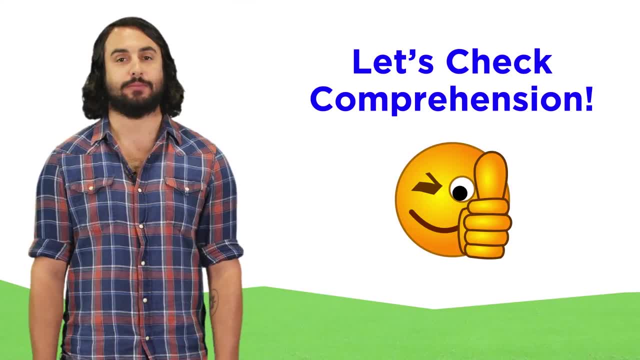 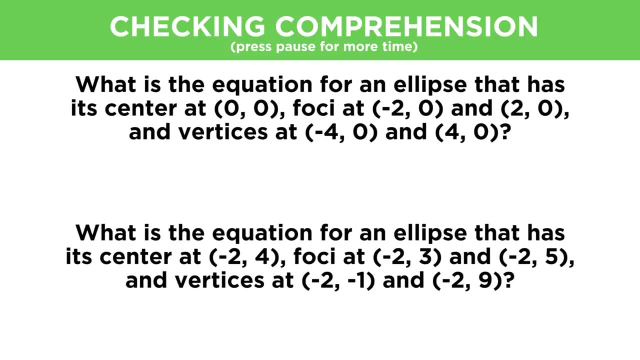 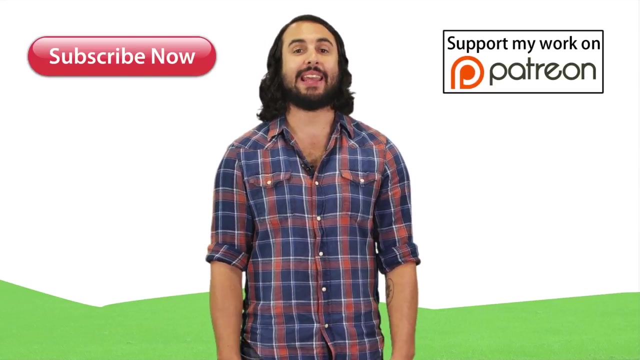 But for right now, we've got a lot more math to cover, so let's check comprehension. Thanks for watching, guys. Subscribe to my channel for more tutorials, support me on Patreon so I can keep making content, and as always, feel free to email me, professordaveexplains at gmail dot com. 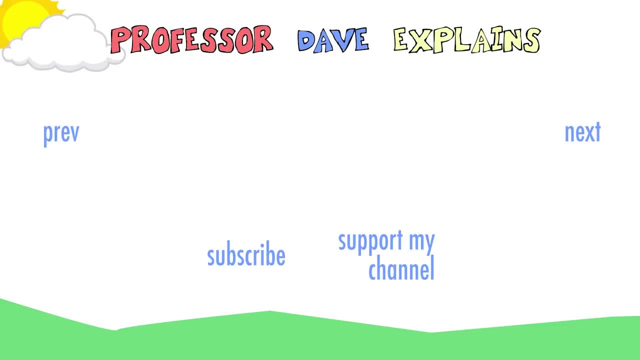 I'll see you next time. 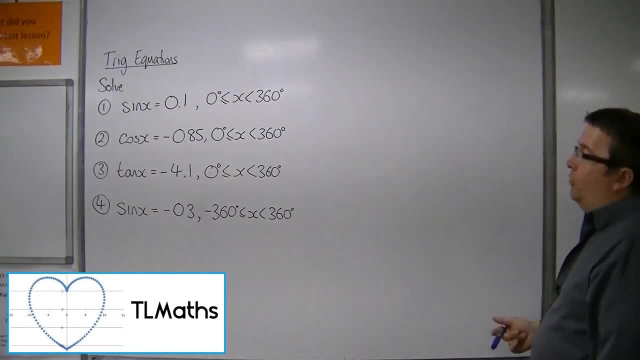 Okay, so in this video we are going to solve these four trigonometric equations. They're all in degrees. 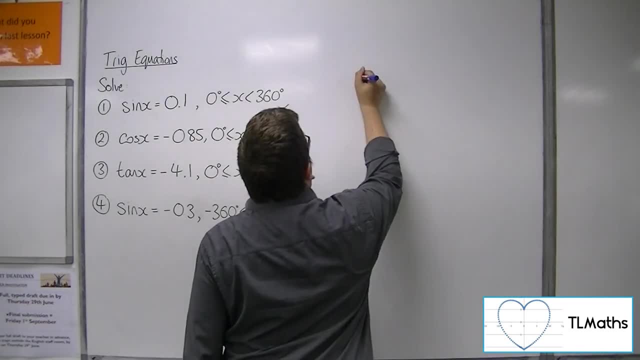 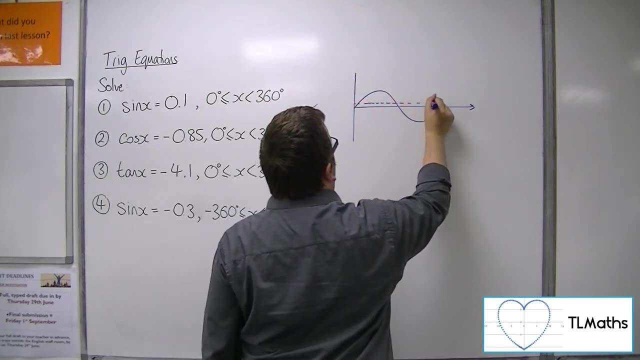 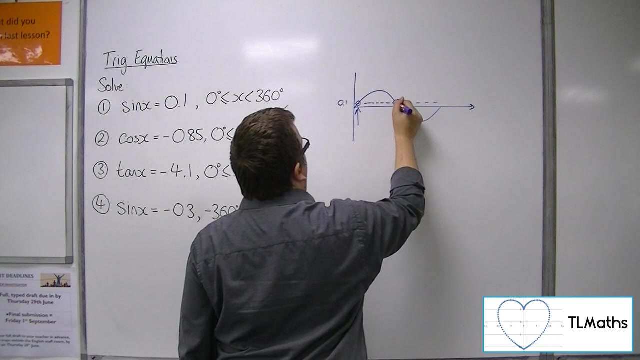 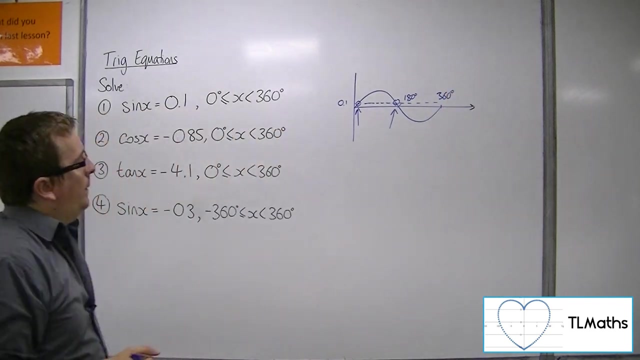 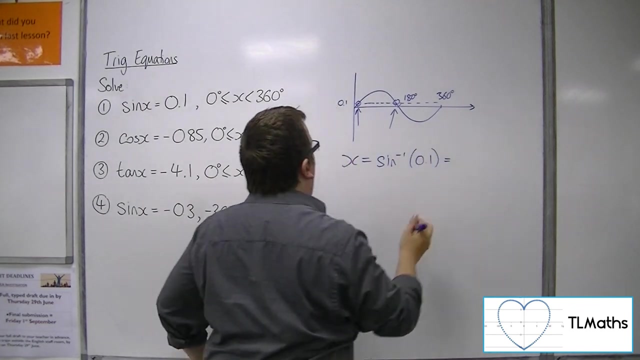 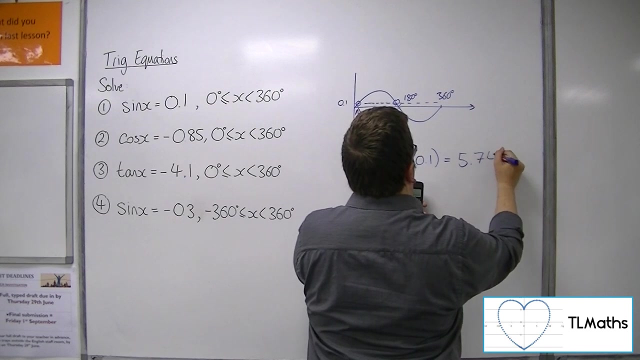 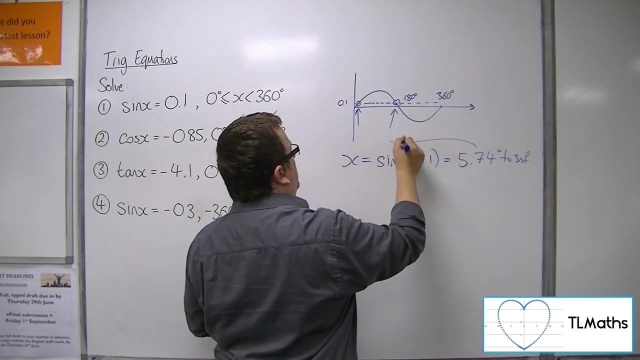 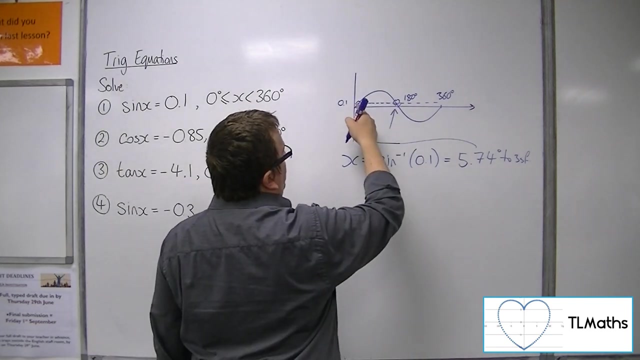 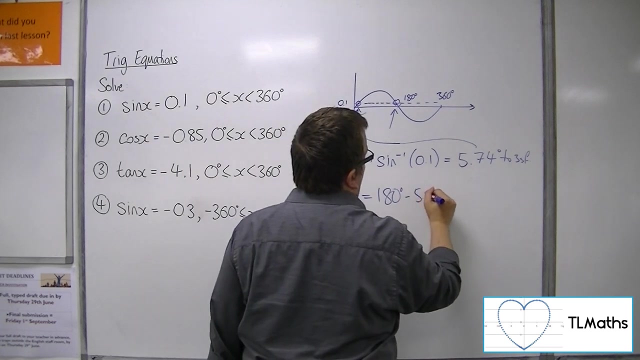 So sine x equals 0.1 for the first one. So we're going to quickly do a little sketch of sine. 0.1 will be about there. Okay, it doesn't need to be accurate. So we're expecting two solutions here. Okay, one there and one there. Now that of course is 180 and there's 360. Okay, so we can inverse sine both sides of 0.1. So inverse sine 0.1 is 5.74 degrees to three significant figures. So that is the first, oh not that one. It is that one there. Okay, that first one. And then the second one, because that's 5.74, that must be 5.74 away from 180. So 180 take away the 5.74. 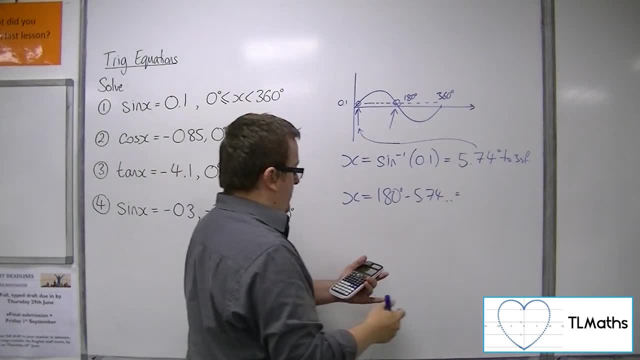 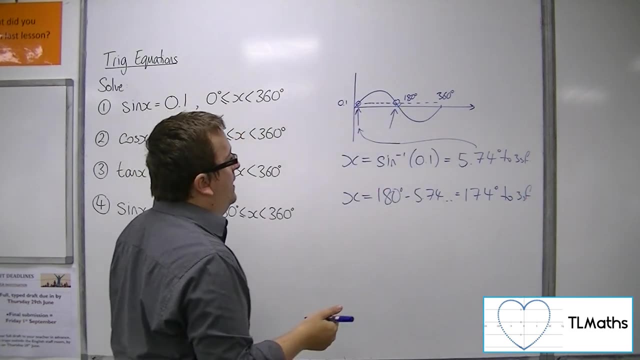 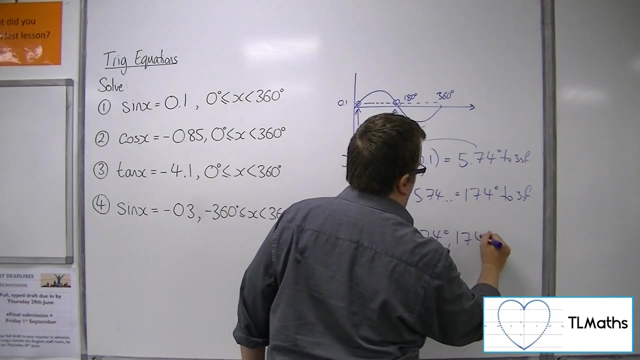 Okay, so 180 take away that answer is 174 degrees to three significant figures. Okay, so these are the two solutions. These are the two solutions to this problem, to three significant figures. Okay. Right, so that's number one. 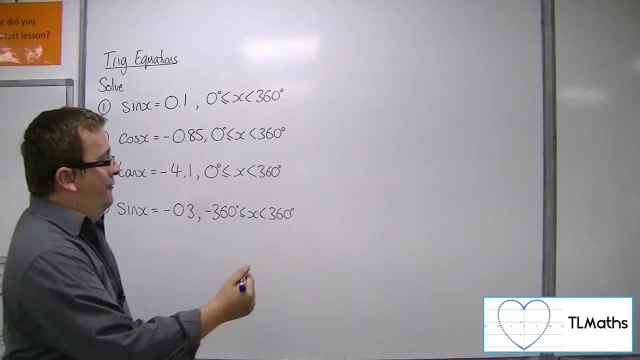 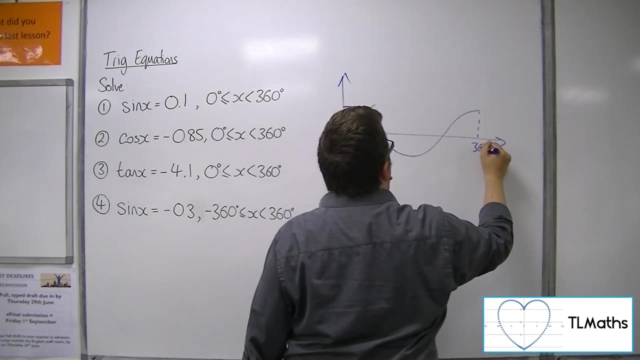 Right, so number two, cos x equals minus 0.85. So sketch of cosine. Okay, once again, doesn't need to be perfect. Minus 0.85, now that's going to be down there.